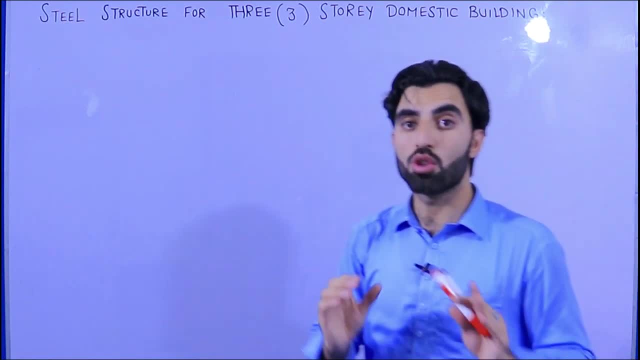 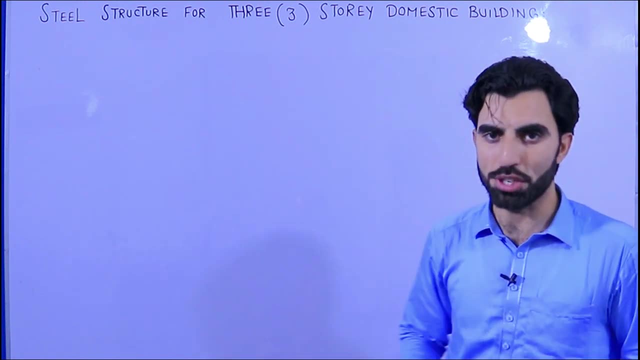 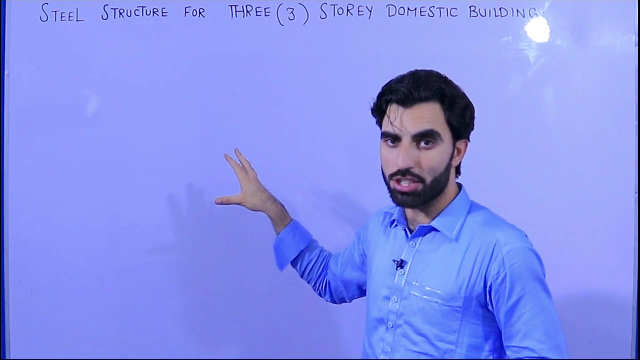 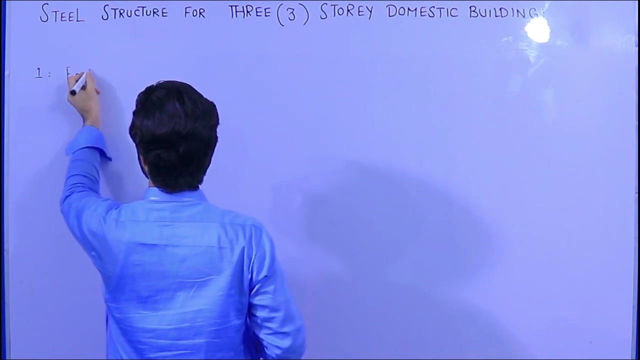 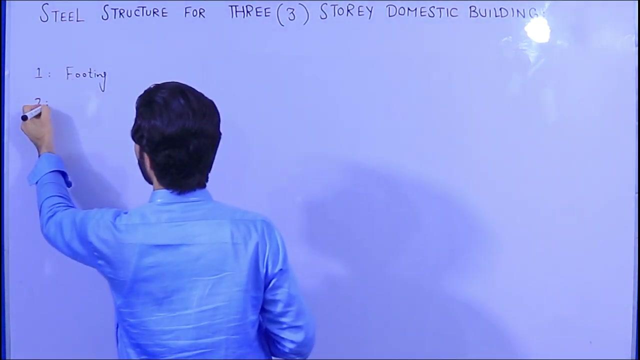 building, not for commercial building, For domestic building, for commercial building. you will see the other steel structure design maybe in next video. Okay, so, guys, this is from my personal experience. So what I will show you in steel structure and this video. the first thing, that is the first, That is about footing: RCC footing, Okay. second, its column: 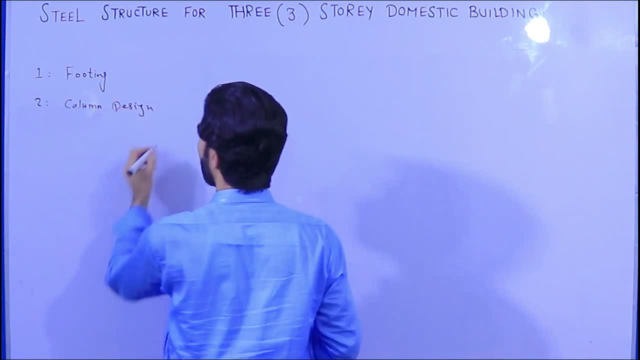 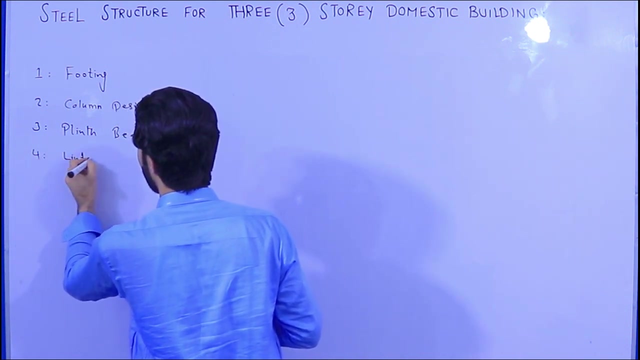 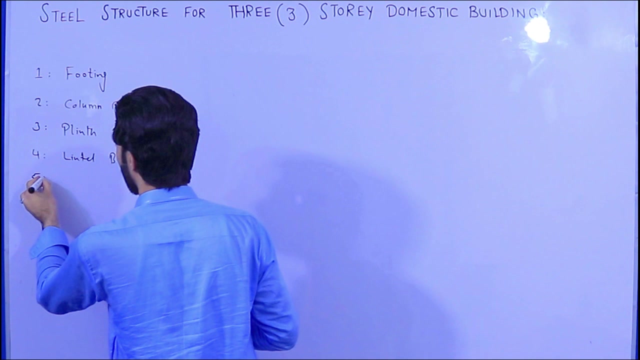 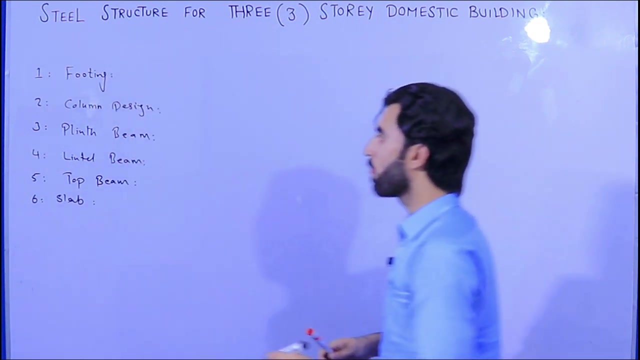 design. Third plant beam, Fourth, lintel beam and fifth that is top beam or you can say slab beam, And the last one is slab, RCC slab. Okay, so the first thing is footing How I did at steel structure. So the first thing is footing How I did at steel structure. 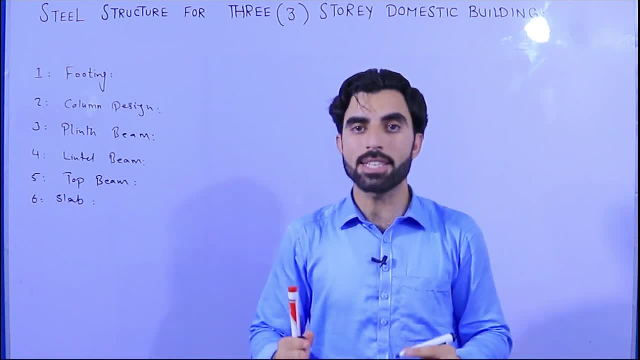 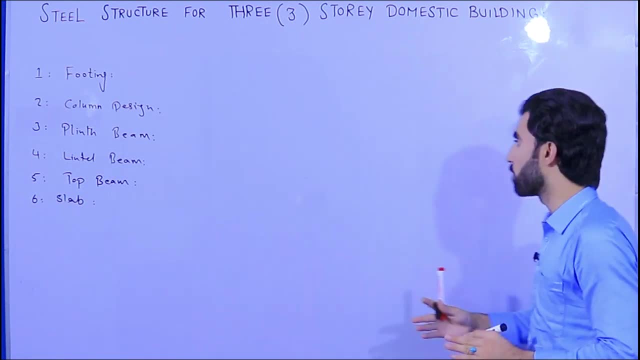 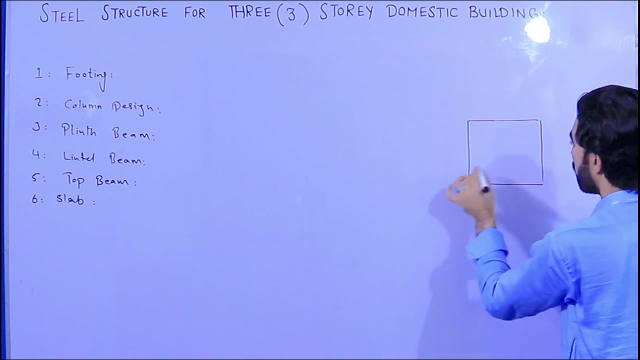 What was the size of footing And its steel structure design, also its depth, Depth of the footing. So, guys, the size of the footing was for domestic three-story building for my client. I will show its videos also, okay, on this channel. The size of the footing was, guys, four by four feet, Four by four feet. 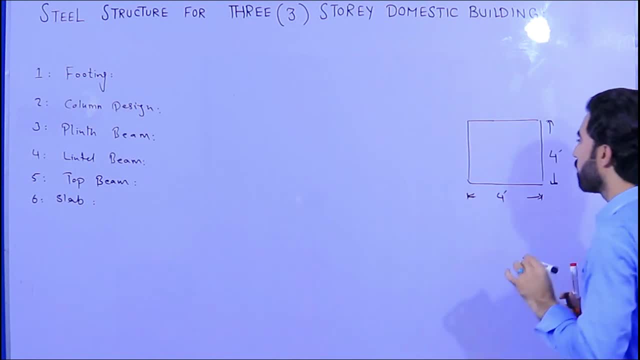 This is the footing size, Right And the depth of the footing was. depth, That was, guys, three feet. Depth of the footing was three feet And its size four by four feet. Now, guys, come to its steel structure design. Its steel structure. Okay, this is for its, I can say, size. 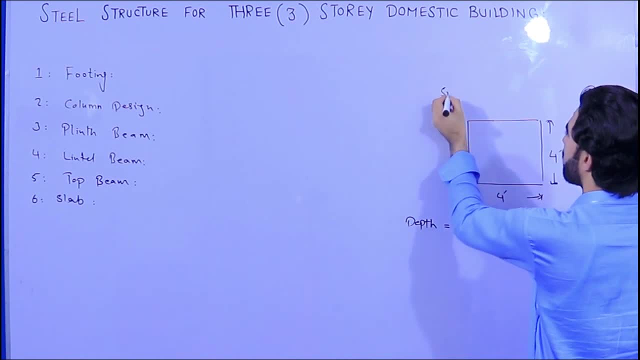 Now, guys, come to its steel structure design. Its steel structure. Okay, this is for its. I can say size And depth, size and depth of footing. Now, guys, its steel structure design. Steel structure for footing. Okay. So, guys, it was like this, as you can see. So here, 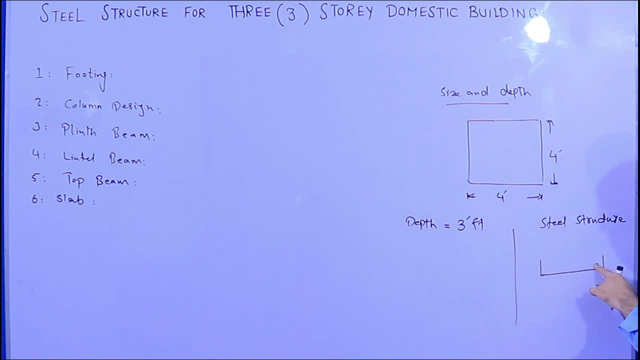 It's steel design, Steel structure design for footing. It's steel structure for footing. So, guys, it was like this. as you can see, this is concrete cover and these are steel bars. so in footing i used 12 millimeter die of steel bar, 12 mm, with the spacing of 150 millimeter. 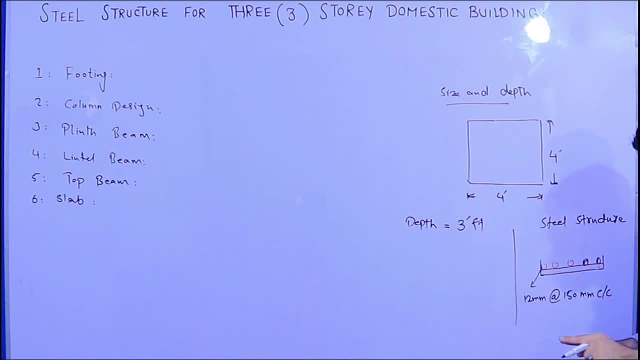 okay, also for main bars and distribution bars. the dia was same for main bars and also for distribution bar, which was 12 millimeter, with the spacing of 150 mm, and the box depth was 300 mm, or 12 inches. it was the depth of steel box, right? so, guys, this is the steel structure. 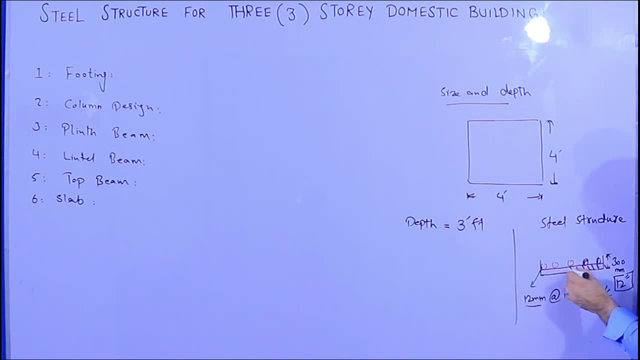 and here, guys, concrete cover. you can see this is concrete cover, bottom and top bar. bottom and top concrete cover was 75 mm and sides cover was side concrete cover was 40 mm. okay, and guys you can see, like this: okay, this is the column at the center and here, guys you can see, these are main bars and also distribution bars. 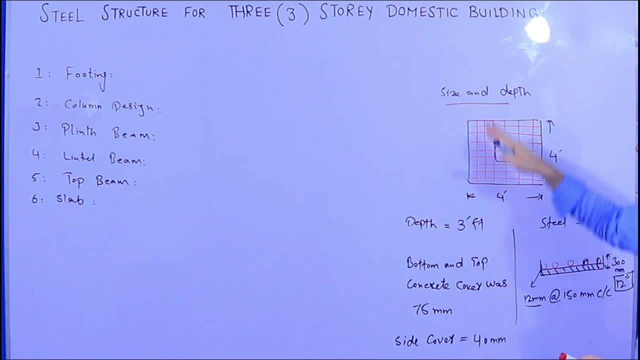 same like this. it was the design of footing size 4 by 4 feet, depth, 3 feet bottom and tops. uh, concrete cover was 75 mm and side cover was 40 mm and i used 12 millimeter die of steel bar with the spacing of 150 for 15 millimeter and i used 12 millimeter die of steel bar with the spacing of 150 for. 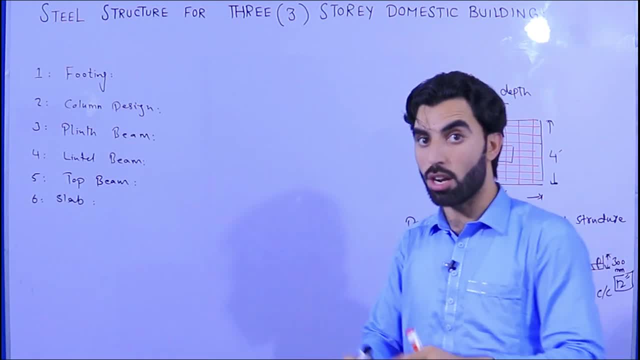 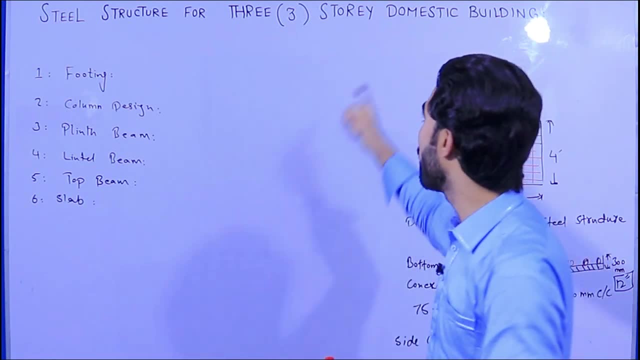 main, and also for distribution bars. the video will be little long, but watch the video from start to end, because this is a special video: full steel structure design for domestic three-story building. right now, guys, for column design. how was the column design? you can see, guys, this is the. 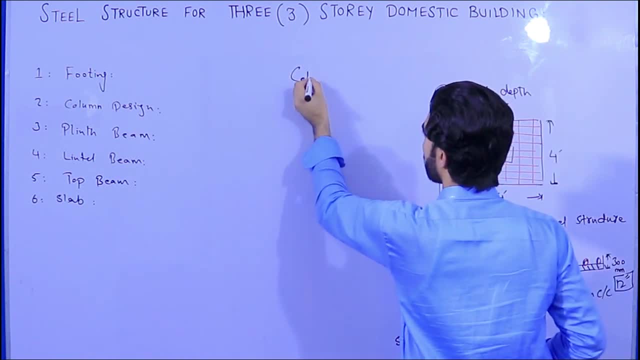 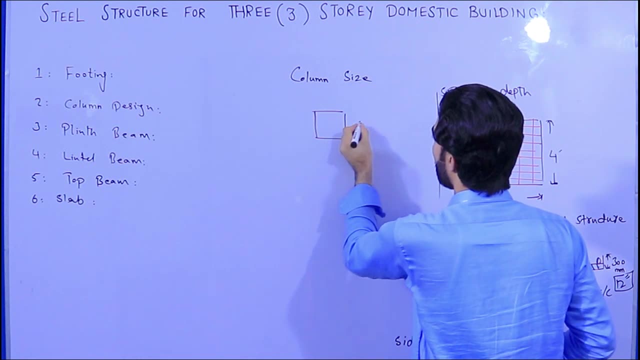 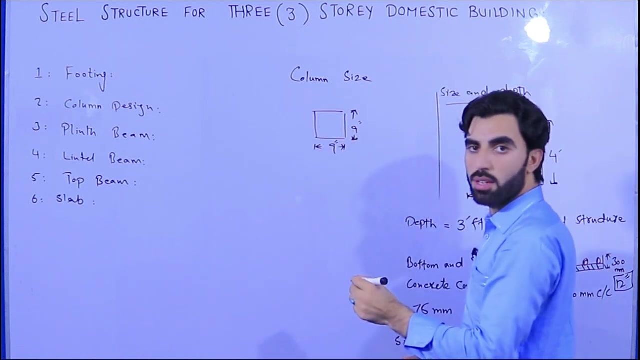 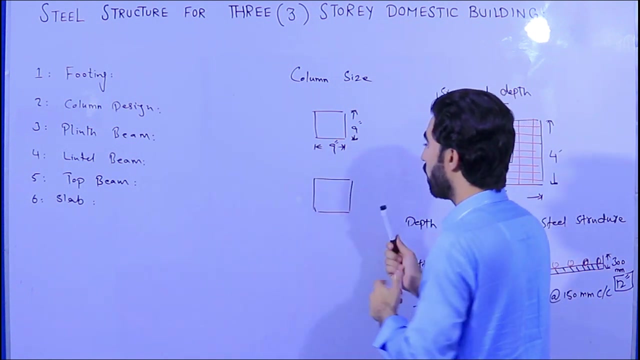 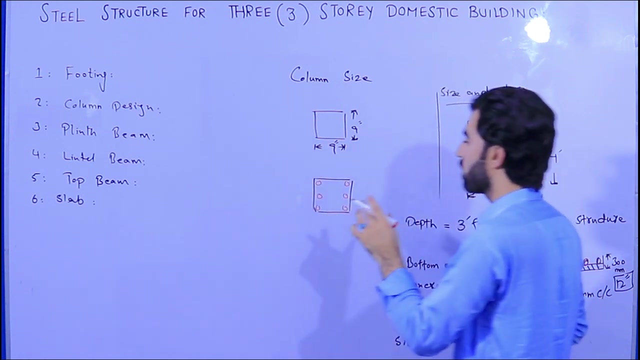 column design. okay. so first, the column size, size of the column was what? nine by nine inches, nine by nine inches, okay, and it's steel structure. I will also show you here, guys, we used here six numbers of steel bars, six numbers of steel bars. NRCC column for three-story: domestic and Gaia. 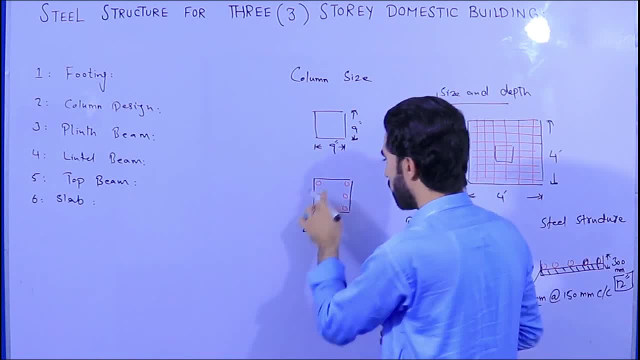 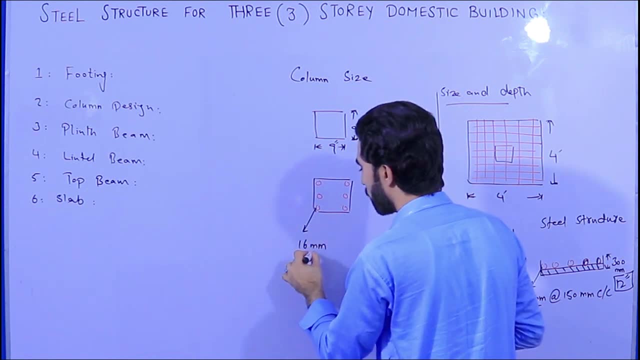 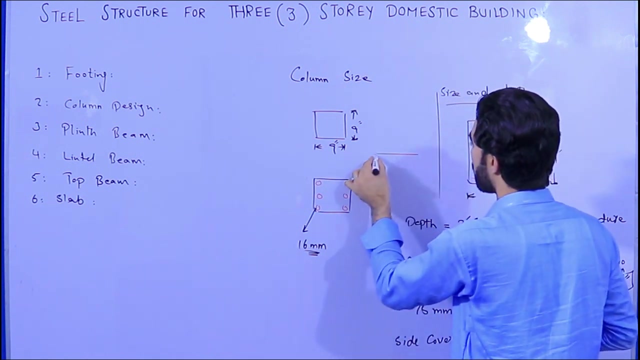 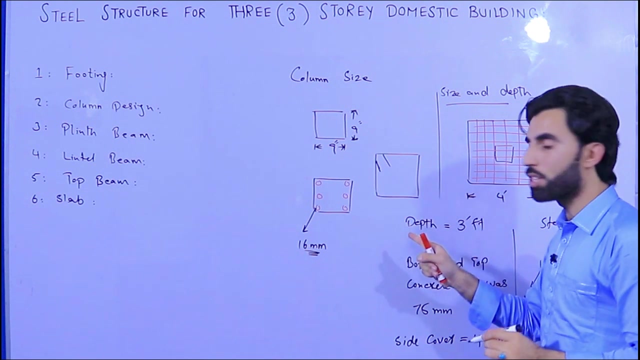 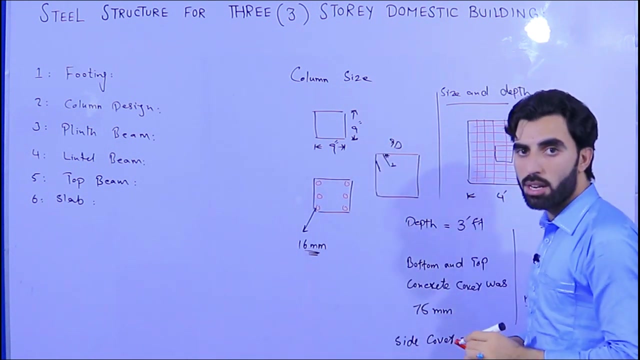 of the steel was for all longitudinal bar. that was guys 16 mm, it was 16 mm, right, and also guys. you can see this is its lateral tie, lateral ties. you can see the hooks were. the hooks length was 90 where it is die of steel bar. okay, and 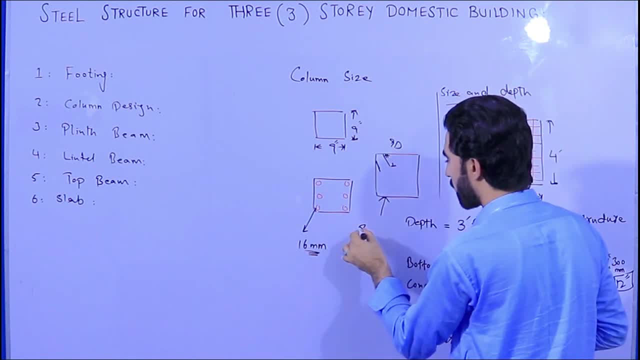 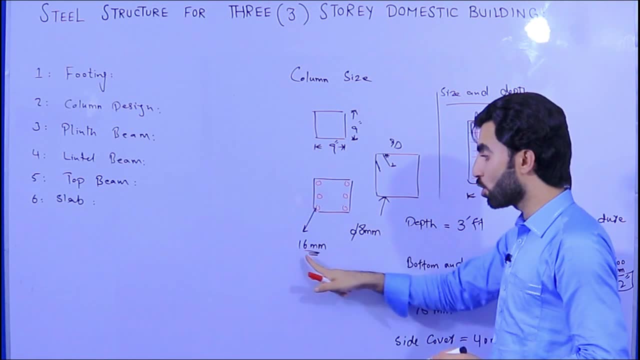 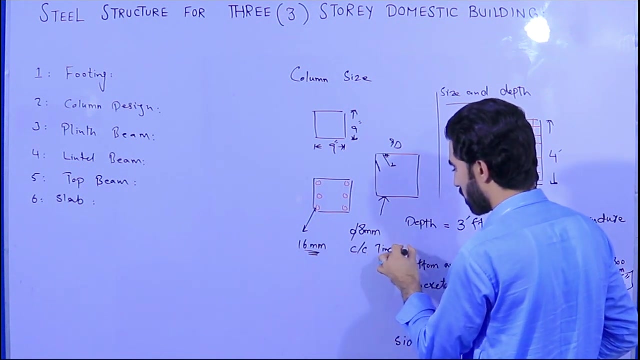 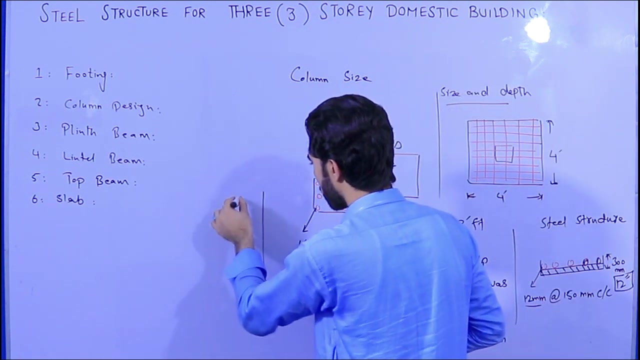 die of the lateral tie was 8 mm. 8 mm diameter of the steel was for lateral tie. that was 8 mm and longitudinal bar 16 mm. with the spacing of guys, seven inches, seven inches. how like this. you can see here. you can see your duck legs. 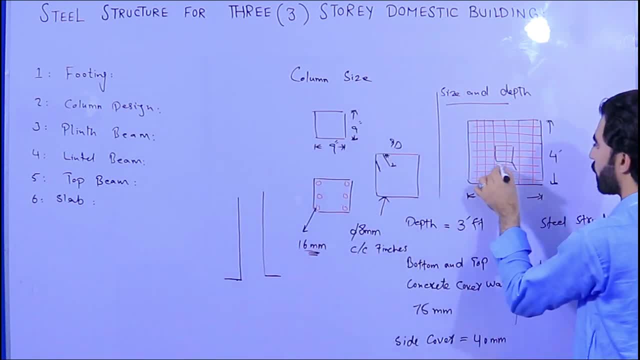 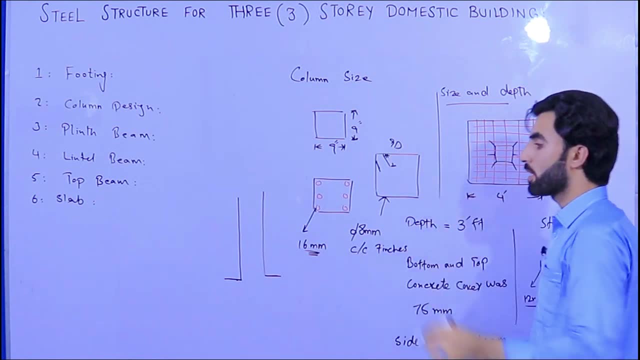 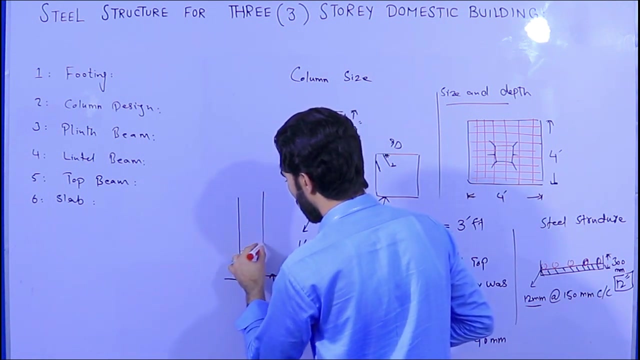 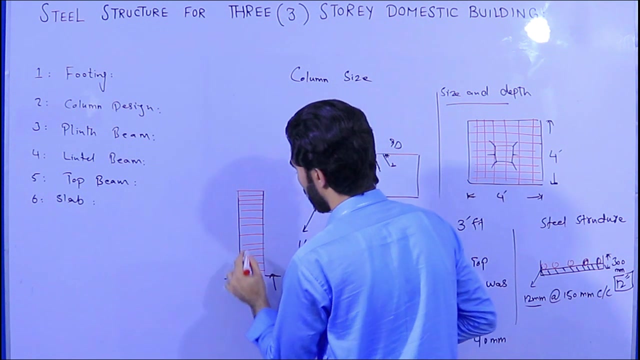 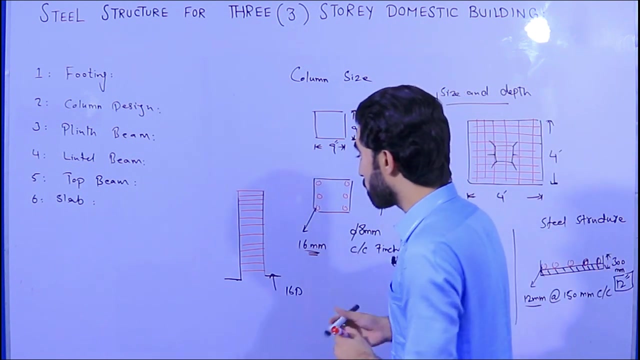 dog leg. okay, so it becomes same like this on the footing, same like this, right, because we have sex numbers and we can get this length with 16D, where this die of steel bar. now, guys, you can see its lateral tie like this, again, with minimum spacing. remember, guys, I did also. I will share its video. okay, so the lateral tie spacing. 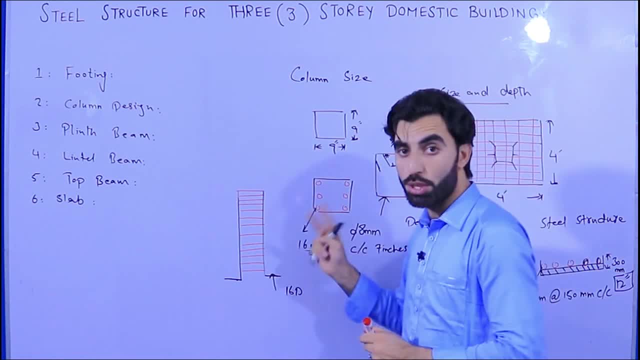 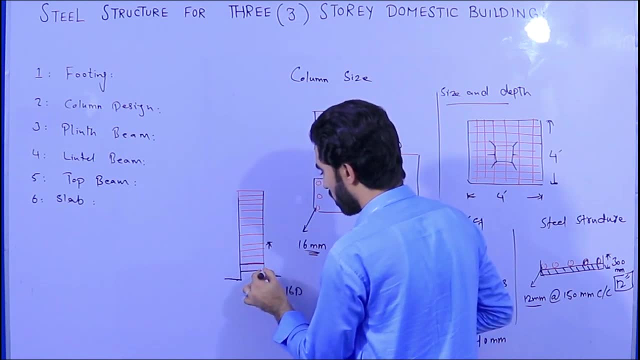 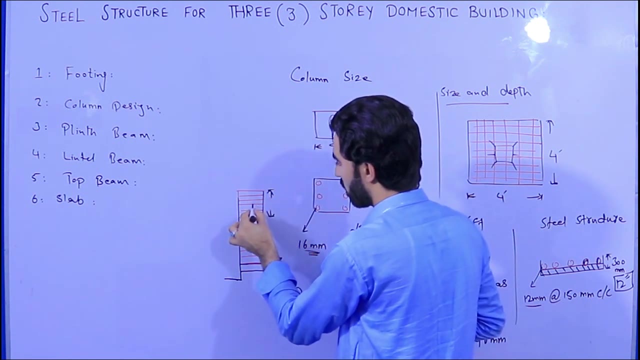 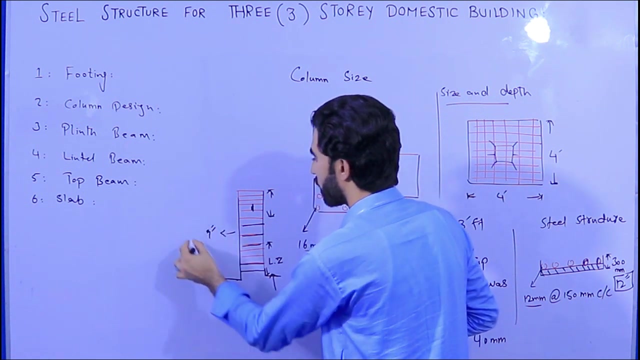 the lateral die, the lateral tie spacing between two lateral tie. okay, that was seven inches at the lapping zone. you can see this is lapping zone, lapping zone and also here with seven inches, as I told you here, but the mid it was about nine inches. the spacing for little ties, remember, and the 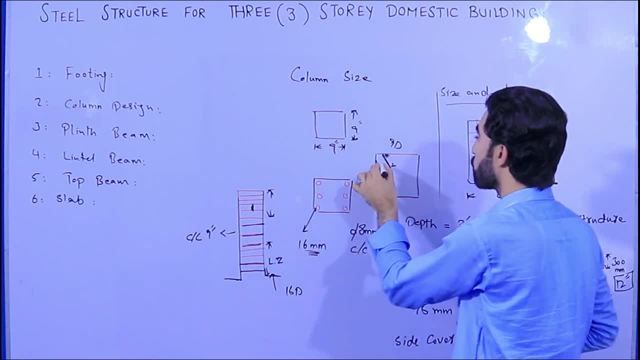 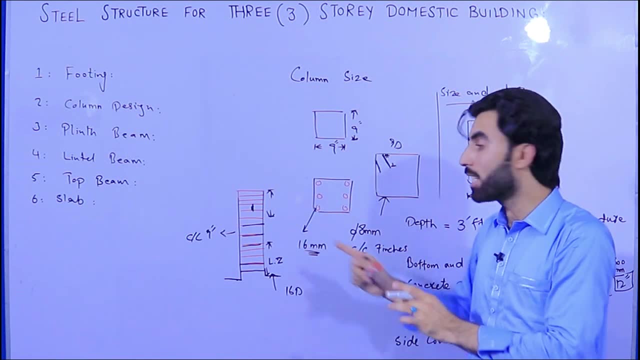 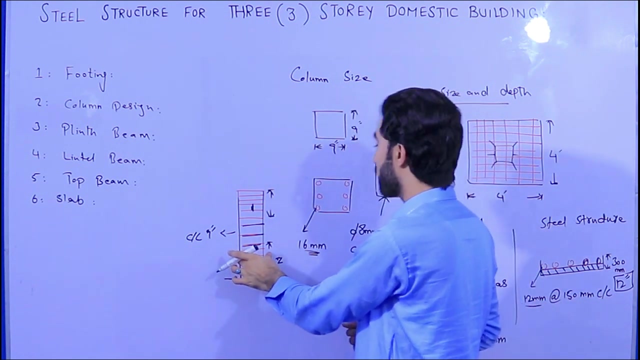 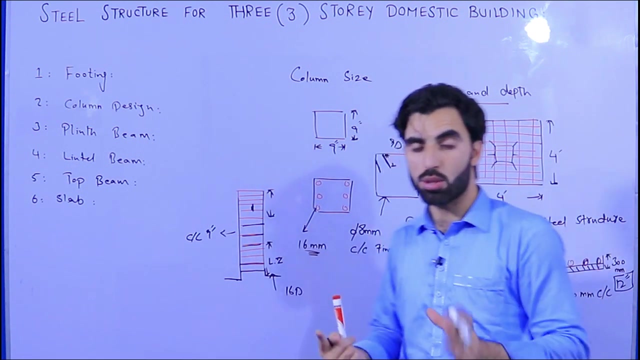 hooks. the hooks should be alternate, not at at one direction. it should be change in different places, so it's depend on you. okay, so at the here, at the lapping zone, its direction should be change the hooks, okay. and also at the top it should be change. at the mid it should be also change, but it should be not in the same. 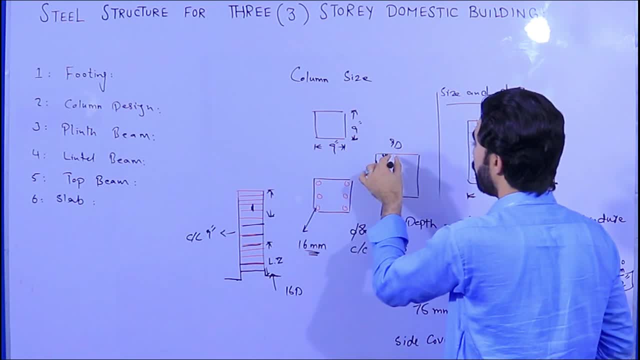 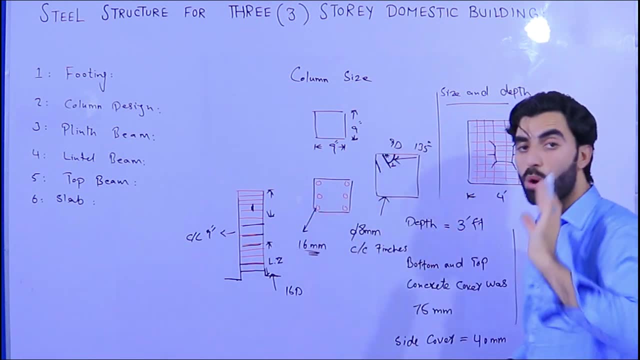 direction. and remember, guys, wait here, we did this angle, angle of hooks, with 135 degree. this is also very compulsory, okay. so, guys, this is the design of column, steel structure design of column. now, guys, come to its plant beam. how we did the design for plant beam, guys? so first I will erase 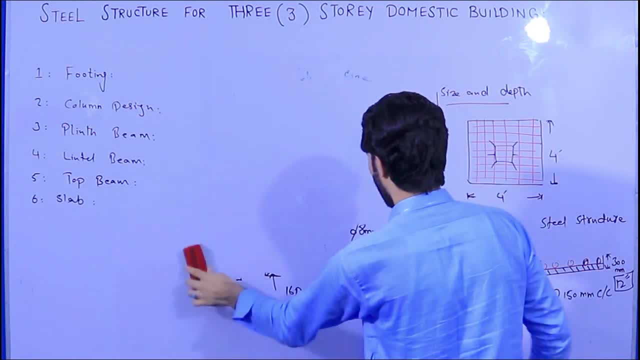 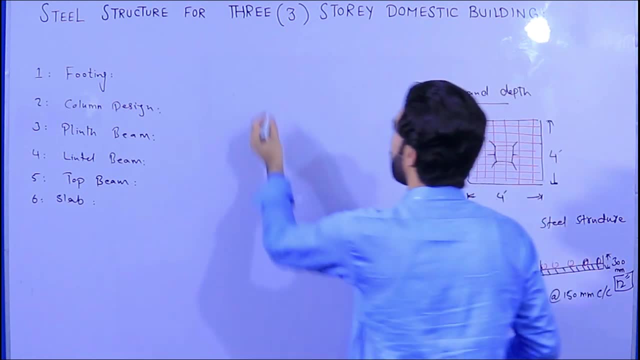 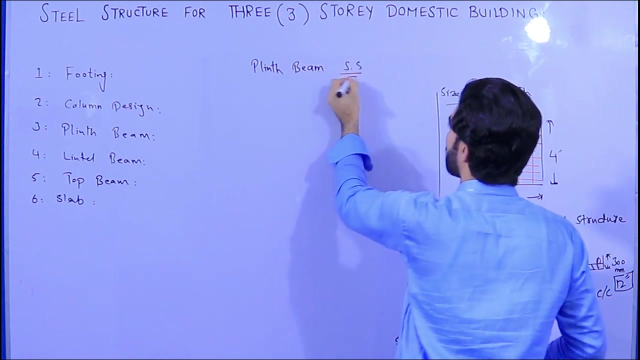 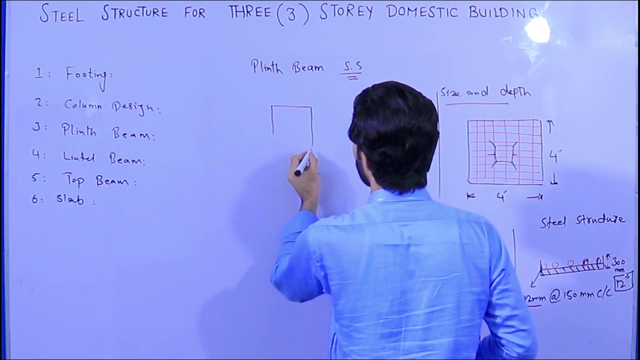 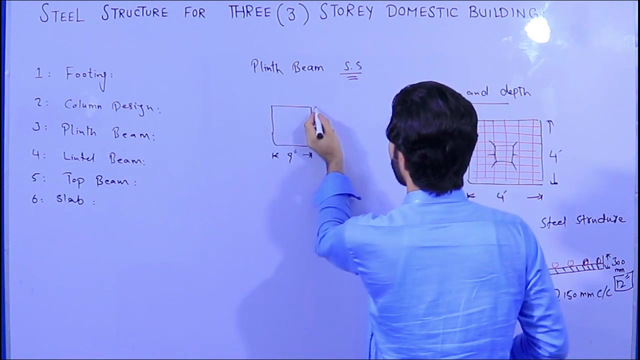 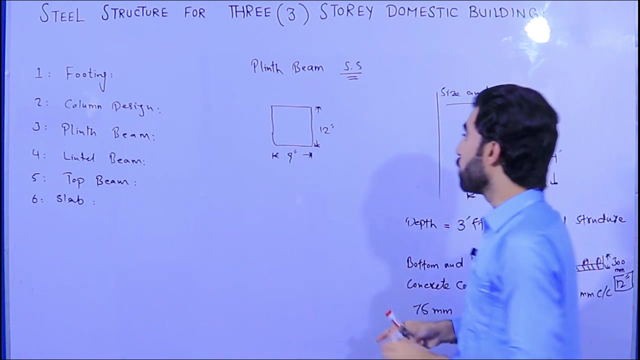 this, okay, if you don't mind. so, guys, you can see here plant beam, steel structure SS. okay, shortcut. so, guys, the size of the plant beam was, its width was nine inches, okay, and it's a depth 12 inches for three-story domestic building and we used here, guys, four. 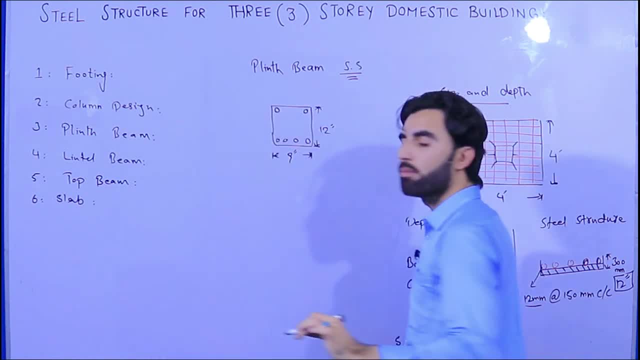 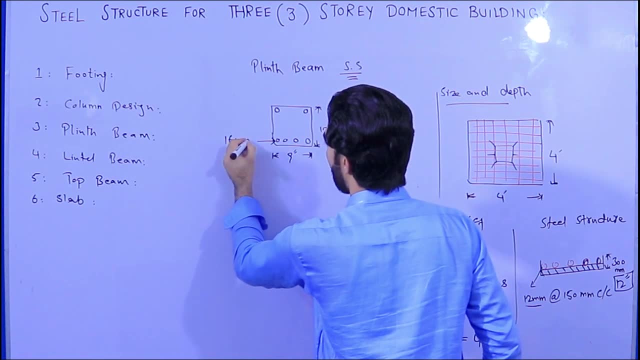 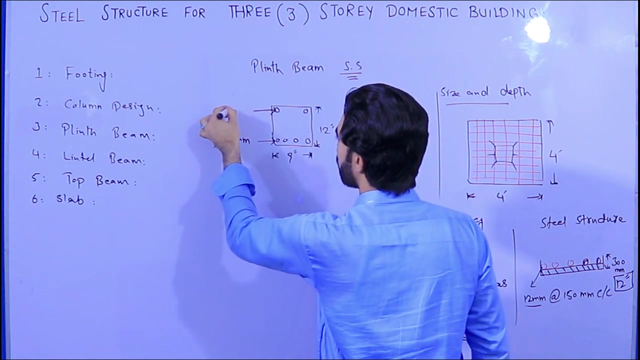 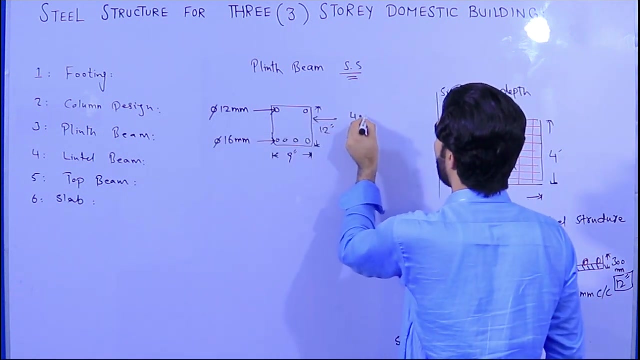 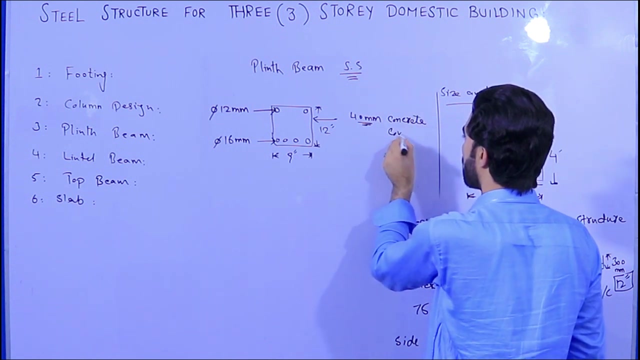 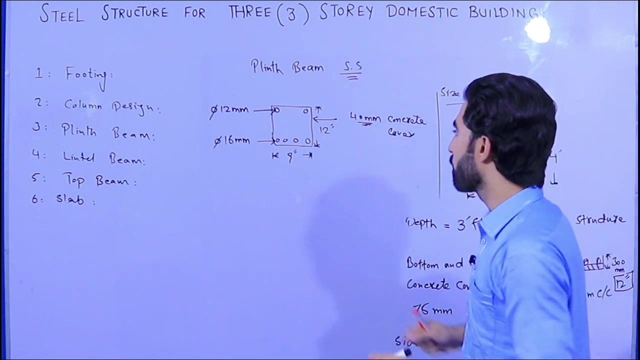 numbers at the bottom and two numbers at the top. the bottom bar dia was 16 mm and and the top bar dia was 12 mm. now, guys, it's concrete cover should be 40 mm concrete cover. okay, now, remember, guys, from 25 to 40 mm. okay, it should be now, it's later, it's you can see. 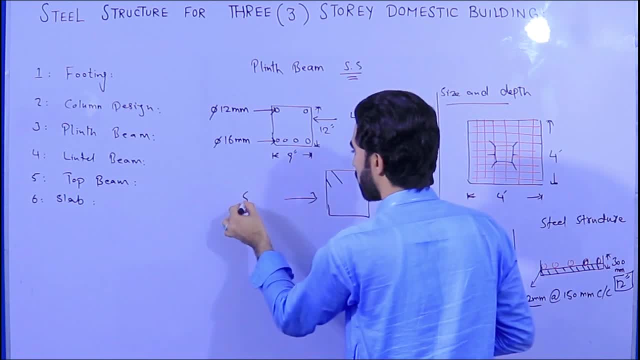 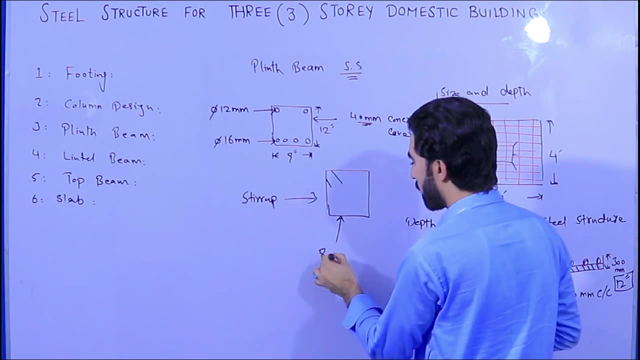 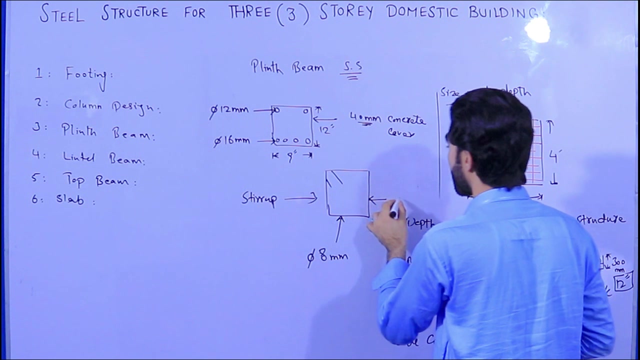 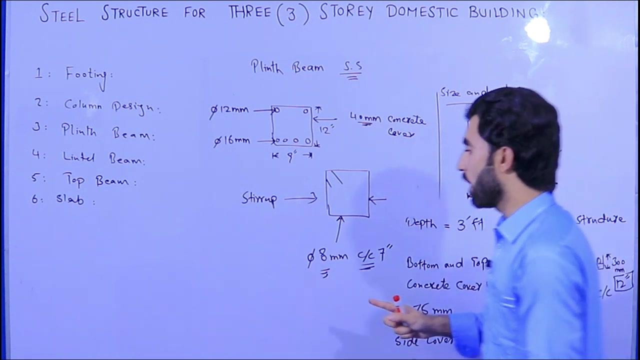 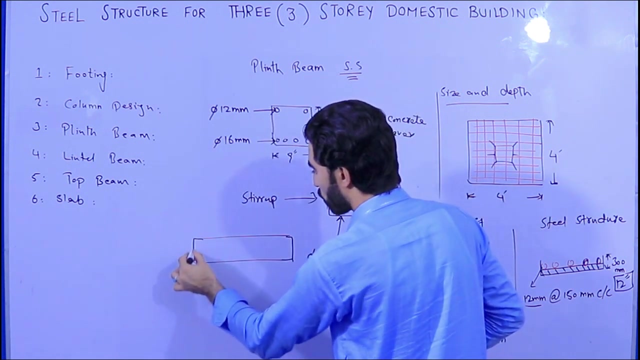 guys, this is its stirrup. so the stirrup dia was this stirrup dia. it was also 8 mm. same for column RCC, column we did with the spacing of again 7 inches, with the spacing of 7 inches also. remember, guys, as you can see, it was also. this is the long section you can see near its support. support is: 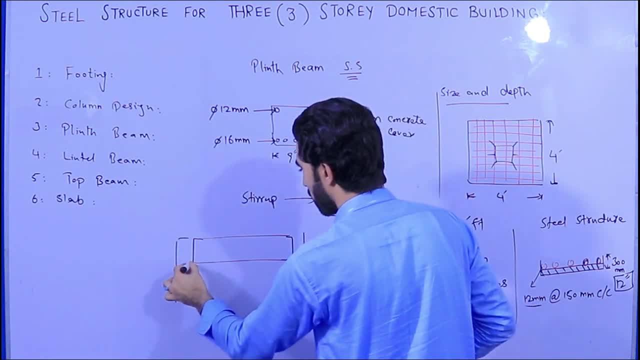 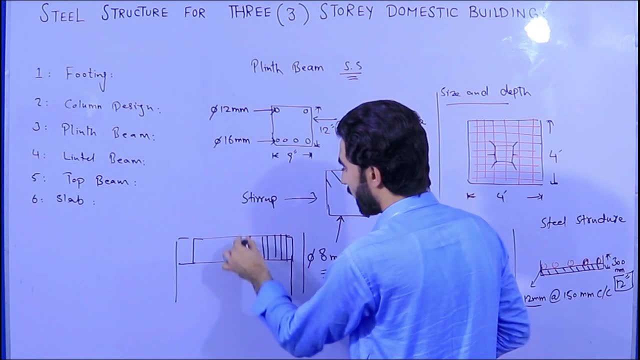 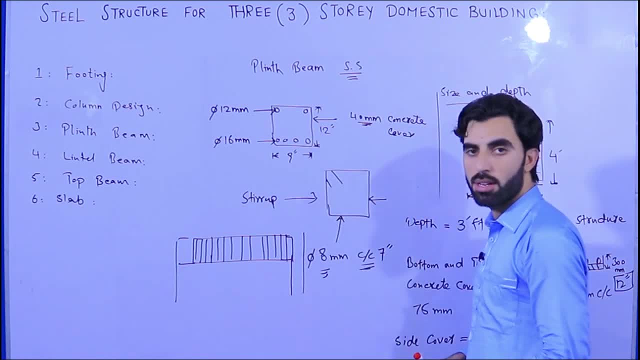 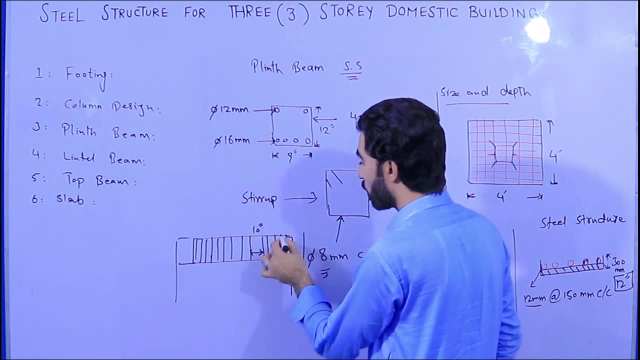 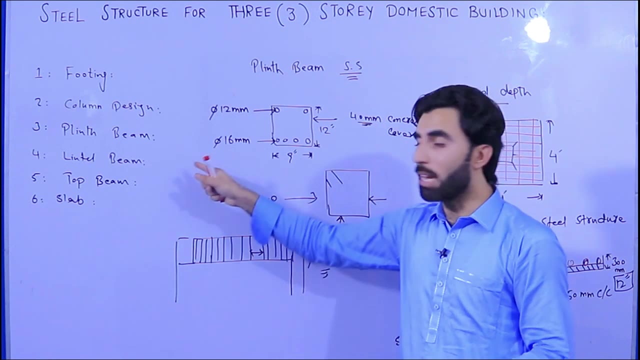 it should be maximum. again, at the end of the support it should be minimum, okay. so here, guys, you can keep about 12 inches, but I did here 10 inches, but near its support it was 6 inches near its support. this is the design of plant beam for this project, which I did in its construction. 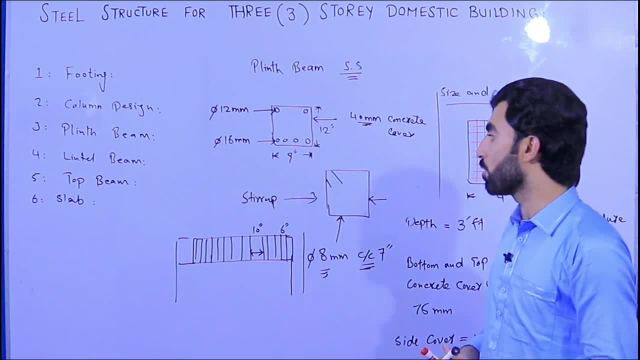 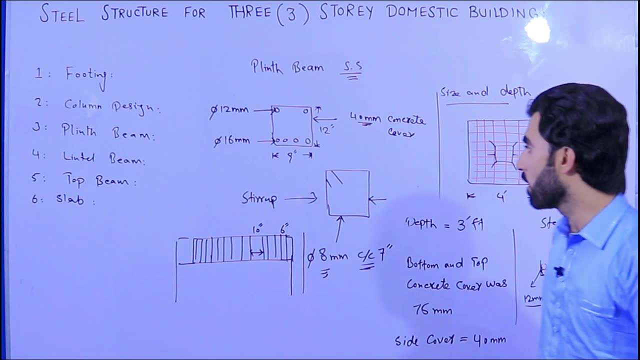 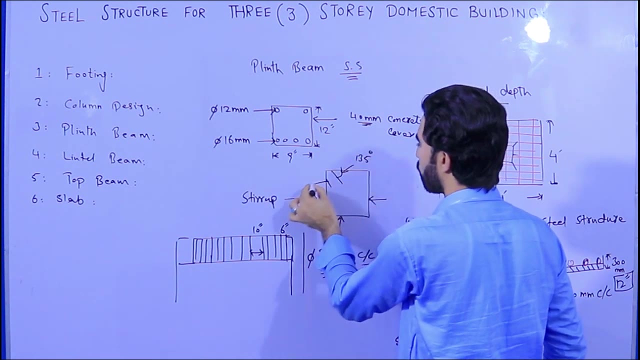 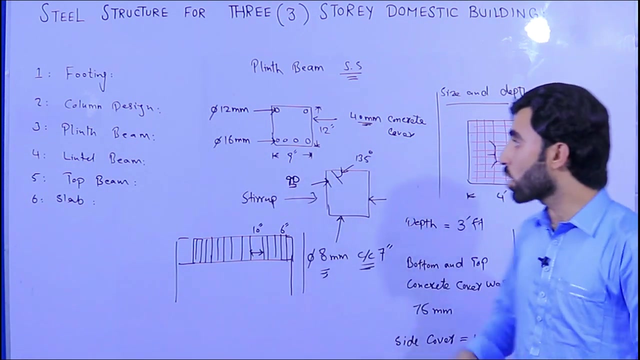 is and progress. this is the design of plant beam, guys. this is the safe steel structure design for domestic building, not for commercial building. now, guys, again, you can see this should be with 135 degree again, and you can get with 90, okay, you can also get 12 D, okay, but I did with 90. therefore, so, guys, this is the design of plant P. now, guys, 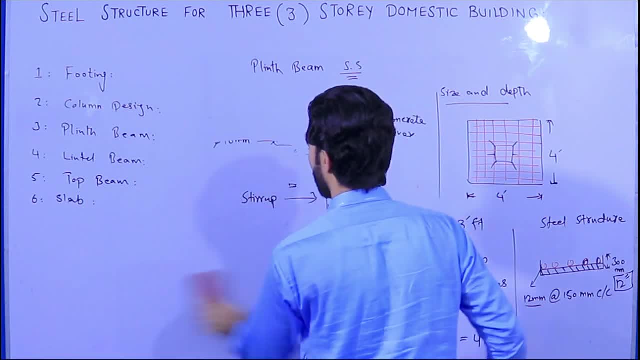 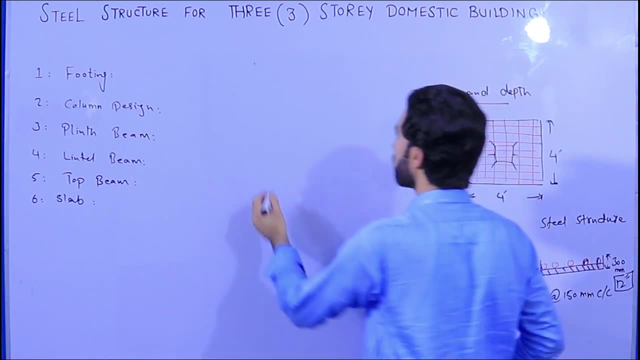 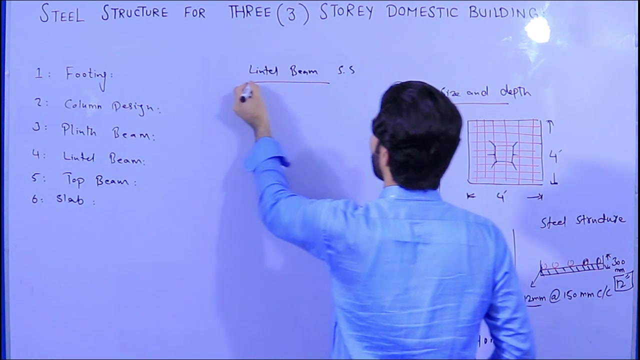 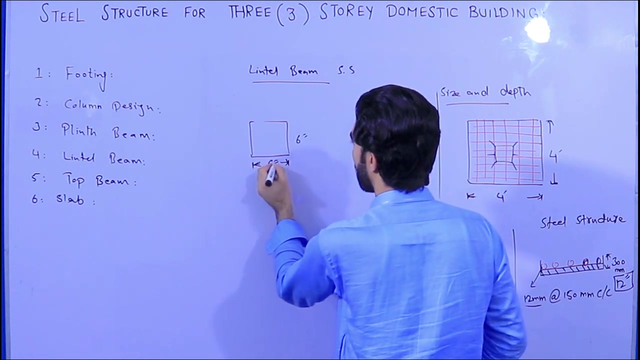 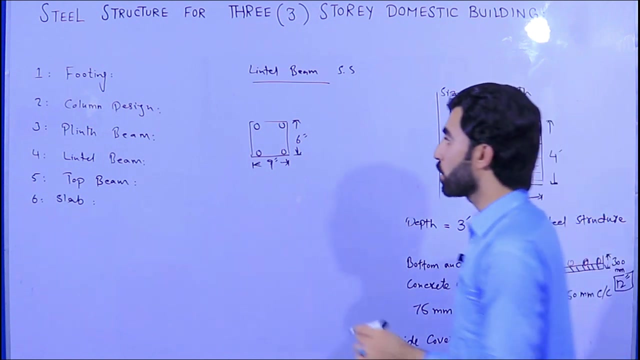 come to its lentil beam. lentil beam steel structure. I did the size of lentil beam, it was 6 by 6 inches. okay. and guys, we used just four numbers of steel bars, sorry, 9 by 6 inches. okay, and we use four numbers of steel bars and top and also bottom bar. dia was 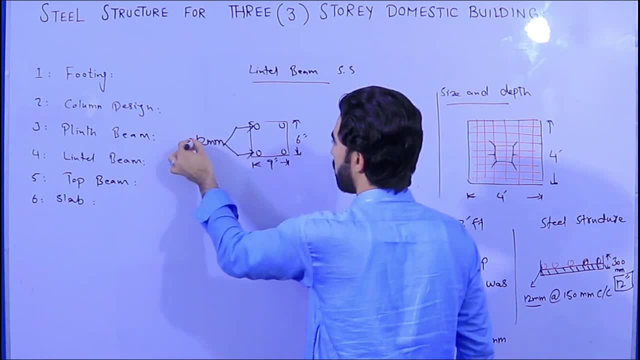 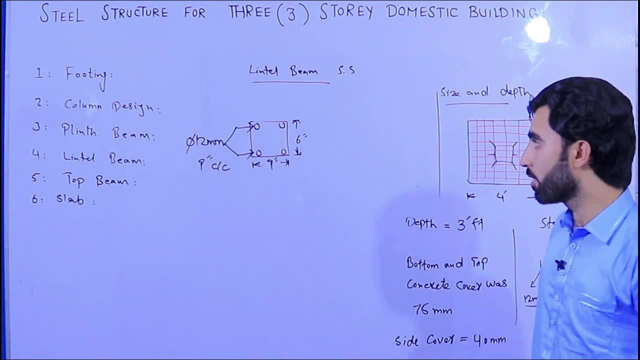 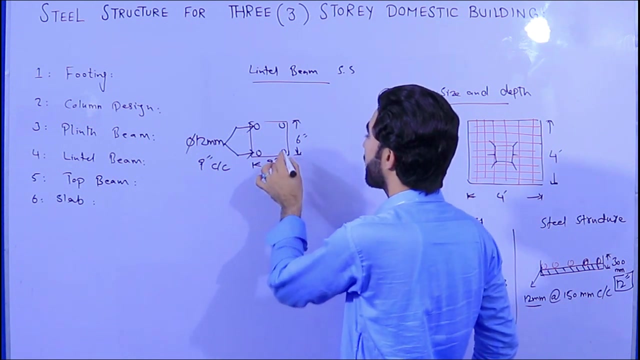 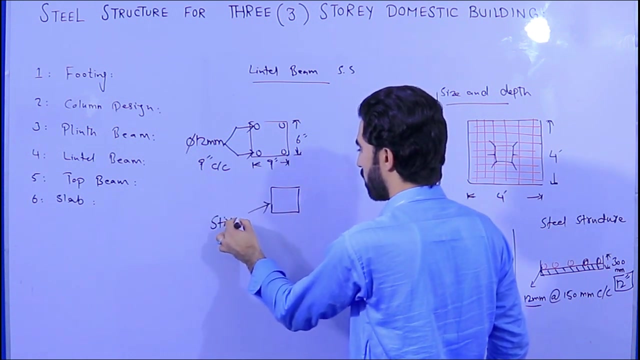 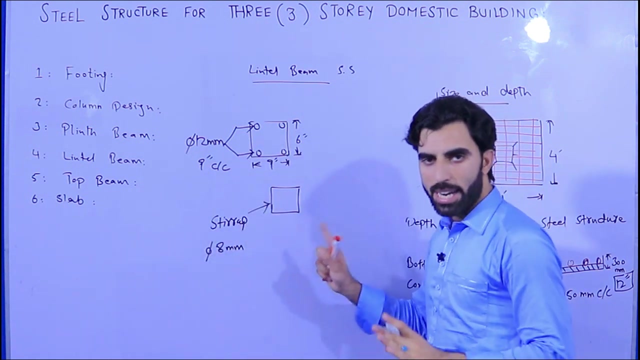 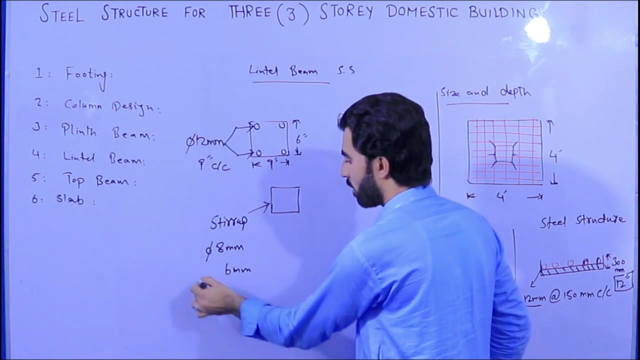 that was 12 millimeter with the spacing of 9 inches for all. okay, this is the lentil beam design and lateral dia was sorry, it's uh, stirrup dia. it was also stirrup dia. okay, stirrup, it was also 8 mm. okay, I did 8 mm because, uh, for all, I use 8 mm, but it should not be minimum 6 mm. minimum is 6 mm. 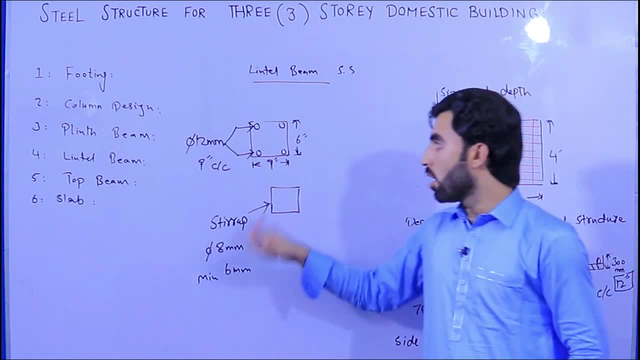 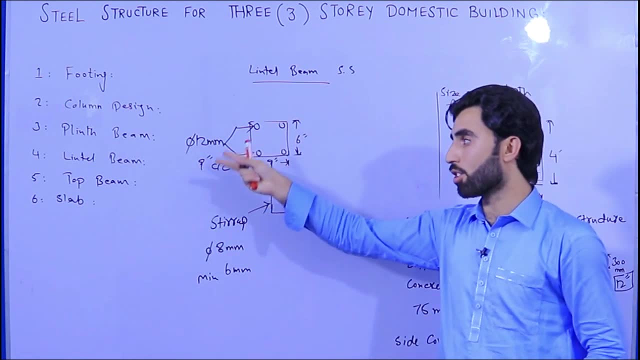 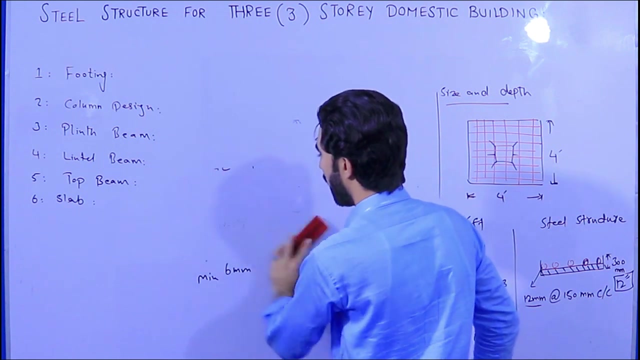 6 millimeter right now, guys, again. okay, also the hooks should be same, like this, like that, as I told you in previous. steel structure design for column. also plant beam. this is the steel structure design of plant beam- uh, sorry, lentil beam. now, guys, we have the design of top beam. 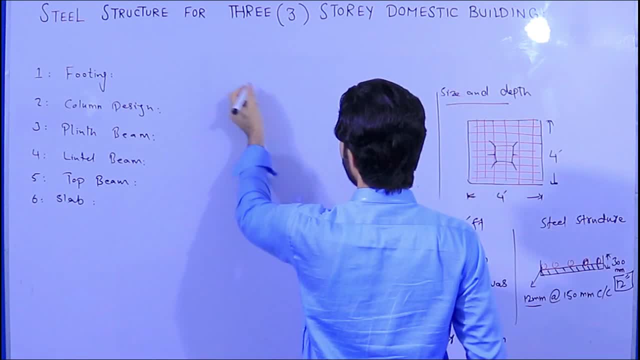 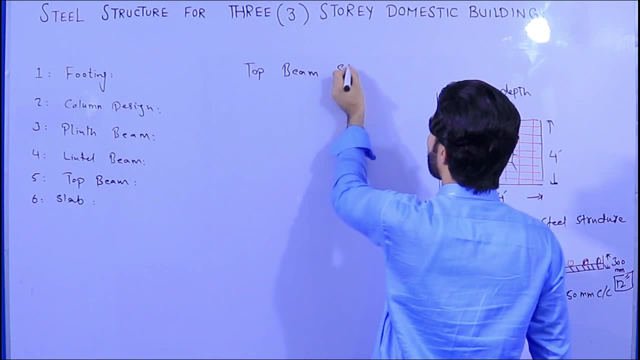 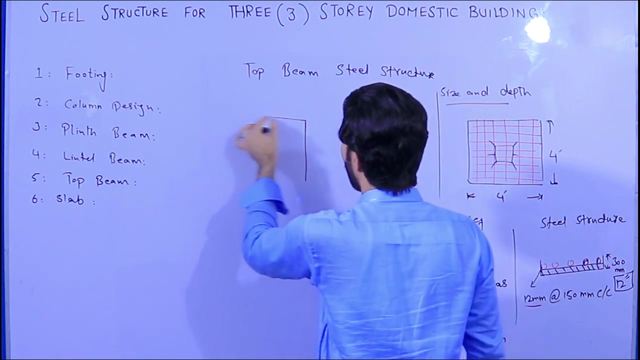 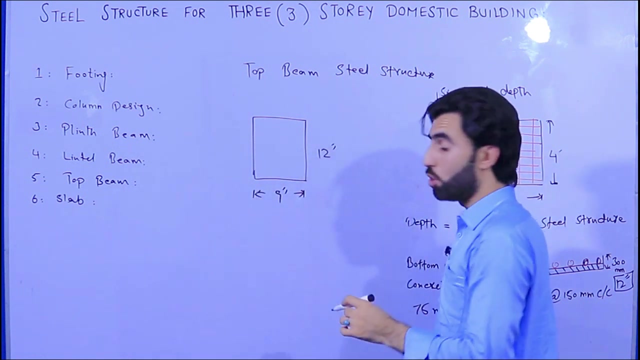 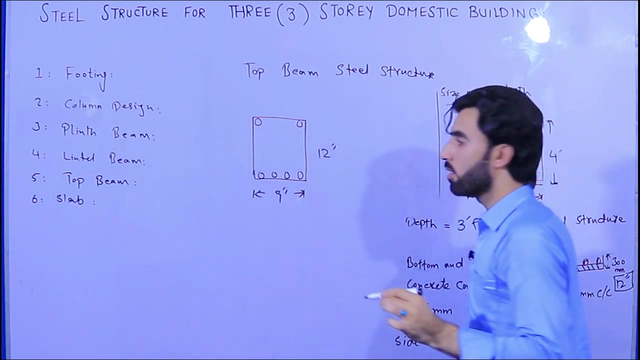 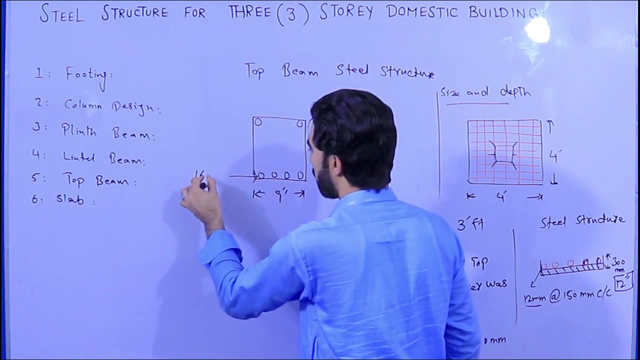 okay. so guys remember, I did the design of top beam, top beam steel structure. okay, here the size of the top beam was 12 inches by 9 inches and we used six numbers of steel bars: four at the bottom and two at the top right. and guys here, at the bottom we used 16 mm dia and at the top we used 12 mm. 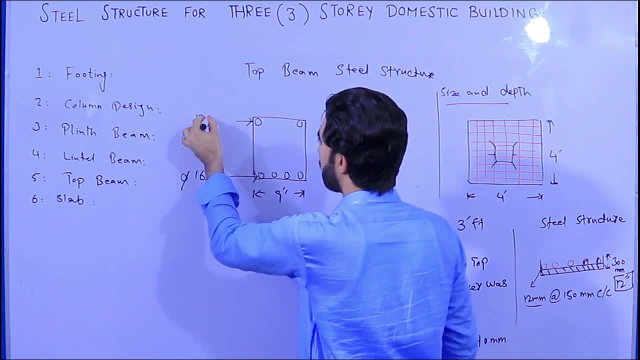 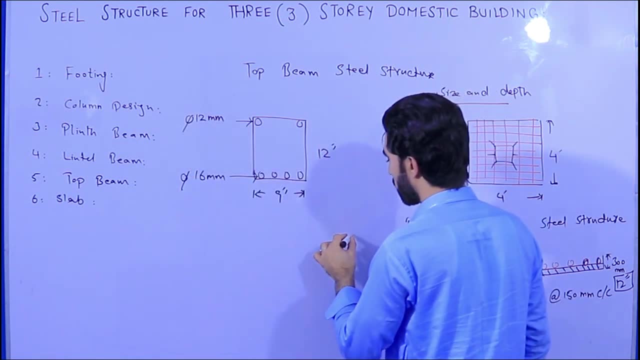 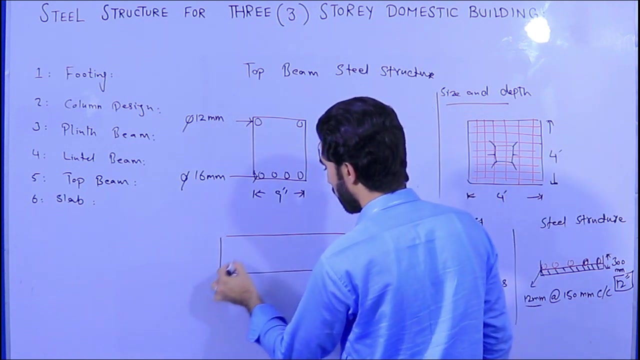 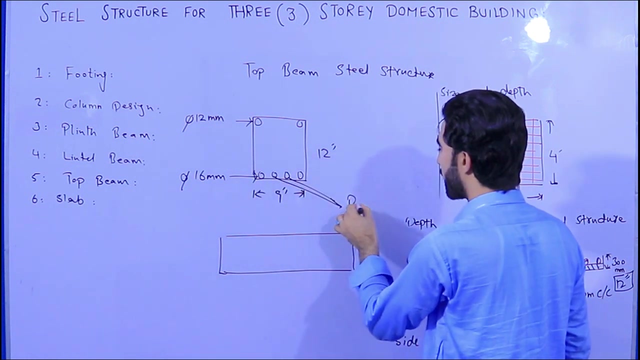 right and guys here: at the bottom we used 16 mm dia and at the top we used 12 mm. right and guys, here I will show you its long section. guys, at long section we have here crank bar, these two steel bars, this one and also this one. this is bent up bar. 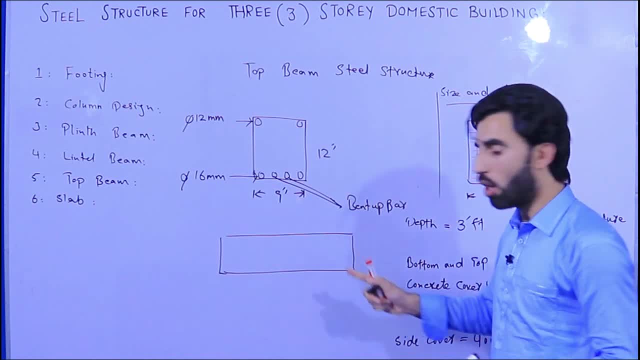 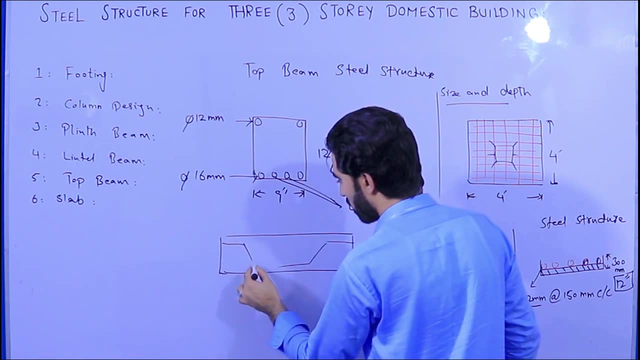 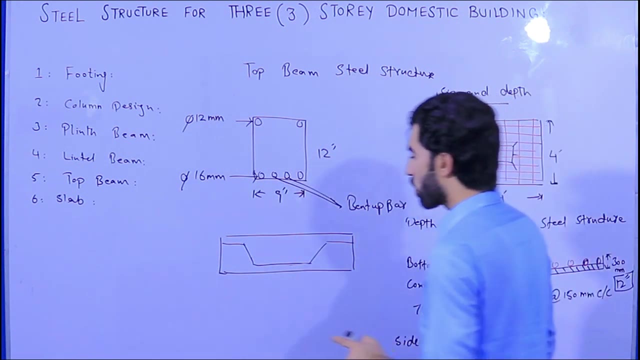 which we bent near at support at the top. okay, same, like this, guys, you can see here like this. it was this right. so, guys, it should be with this: angle should be 45 to 60 degree and the bar should be bent with the length of L by 4, and I did with L by 4.. L means full length of beam. 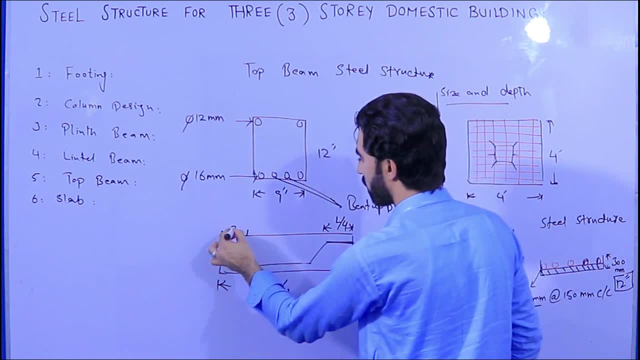 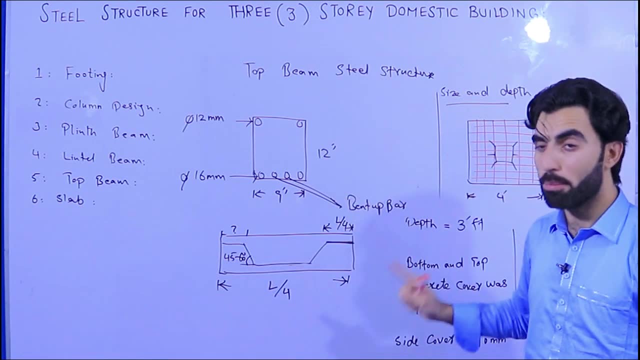 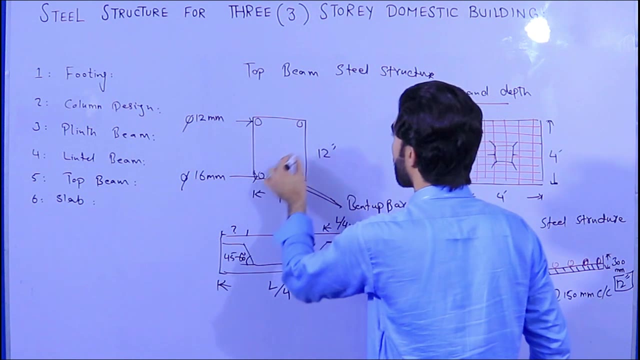 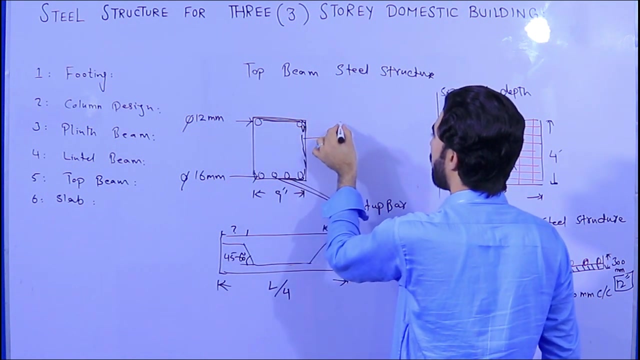 so full length divided by four, then we can get this length. so this length should be crank bar bent up part. remember this point and I did this design for three-story building. guys, concrete cover was concrete cover. as you can see, this is concrete cover. okay, so it should be about 25 to 40 mm. 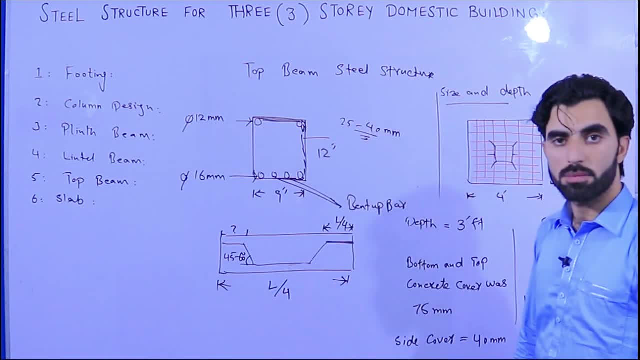 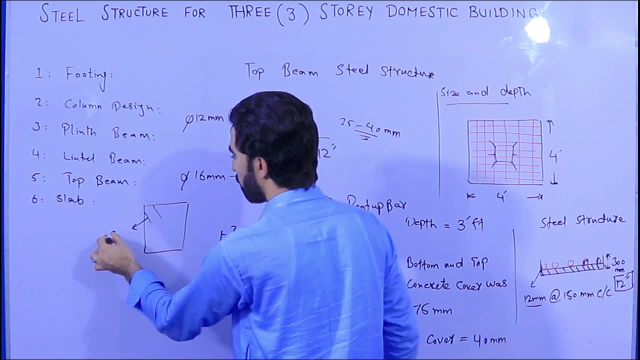 this is concrete cover and I canONEM has arranged it, so that's why it is called a darach Prest disco. so without emotion, people can never do their own job. concrete cover right. and also guys come to its lateral tie. same hooks should be 90 angle. should be 135 degree and i did okay. and the leg, the stirrup dia: it was 8 mm, with the spacing of spacing of 7 inches near its support with crank bar. okay, to the crank bar, it was 7 inches, okay, but at the mid it was going to the 10 to 12 inches, but i did with 10 inch spacing. 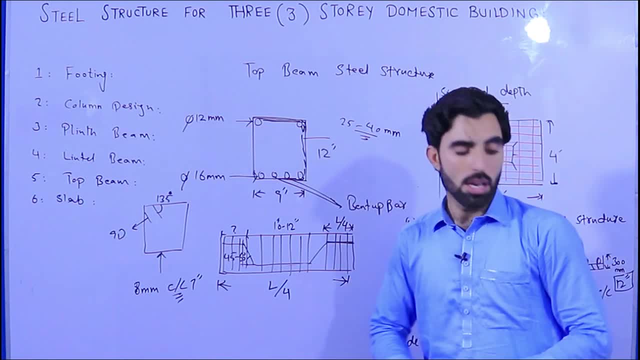 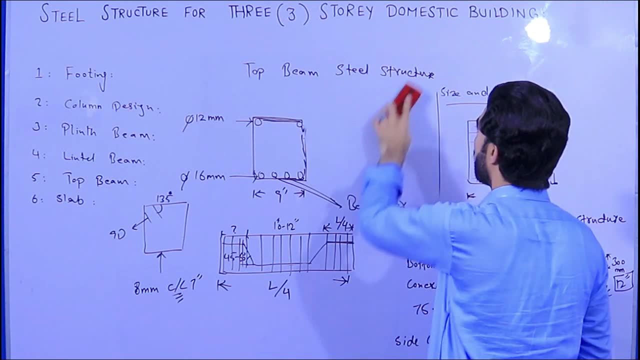 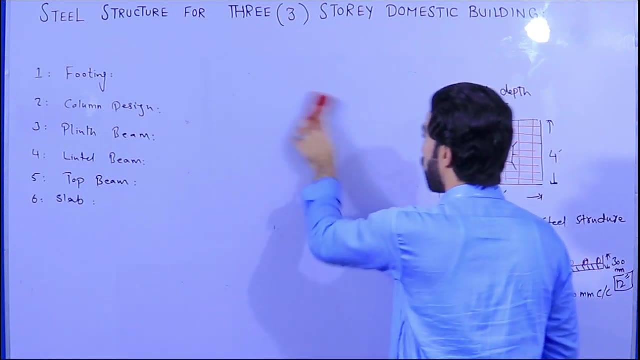 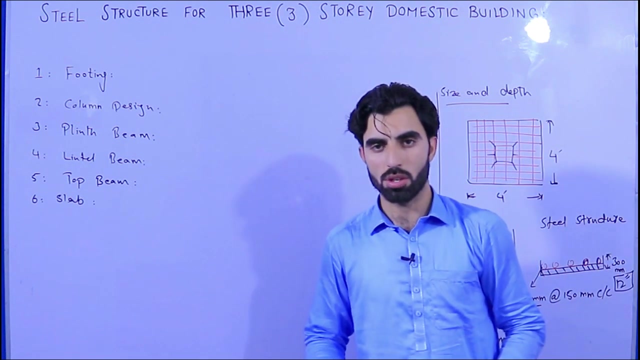 also remember this point for top beam. now, guys, come to its slab steel structure design. now, guys, you will have a question in your mind that from where you did this design, this is: i did more projects. okay, so this is from my personal experience and also from my research. okay, and next video are maybe after some videos, i will show you from where i 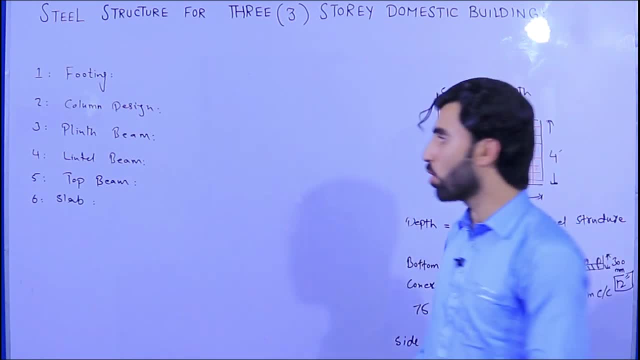 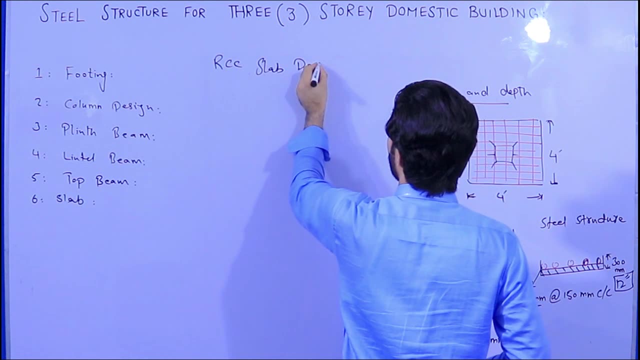 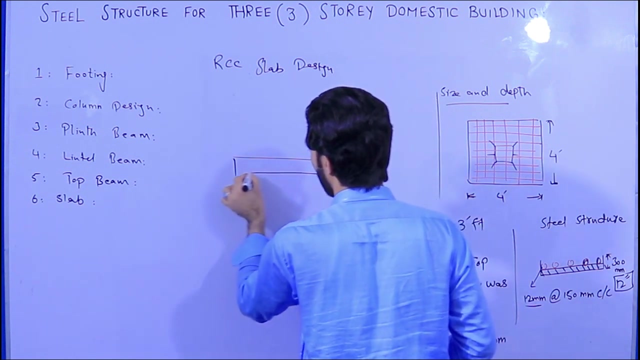 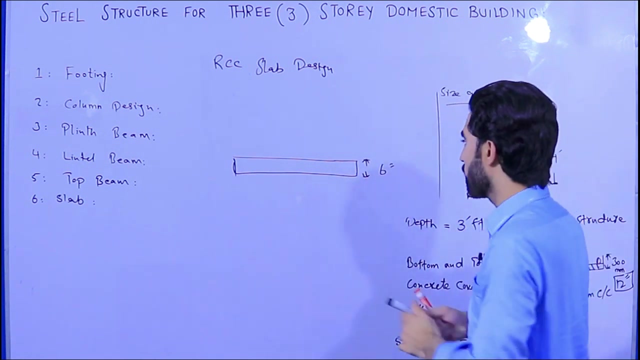 got this knowledge which i'm sharing the front of you, okay. so, guys, come to slab. the last one is slip, rcc slip. so, guys, you can see this is slab. okay, thickness of the slip was six inches, i decide six inches. and here, guys, you can see the bars. 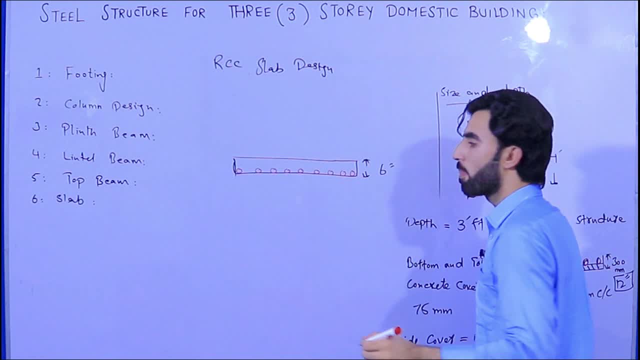 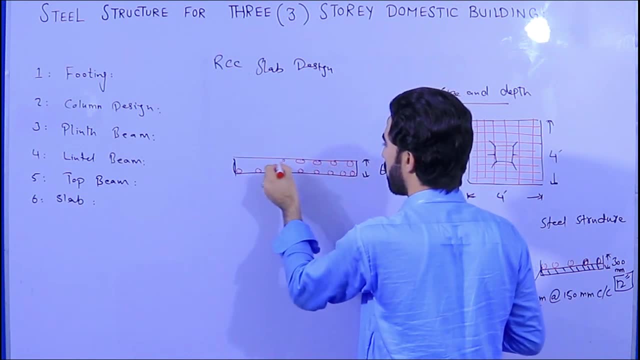 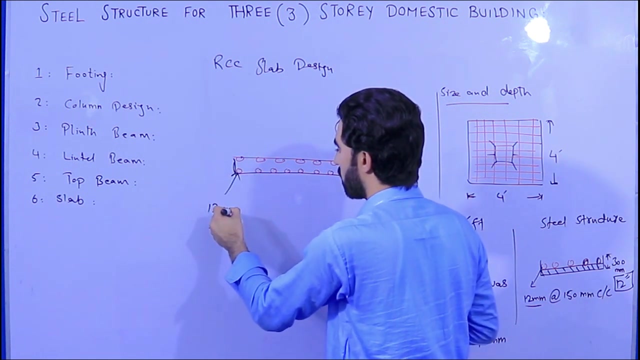 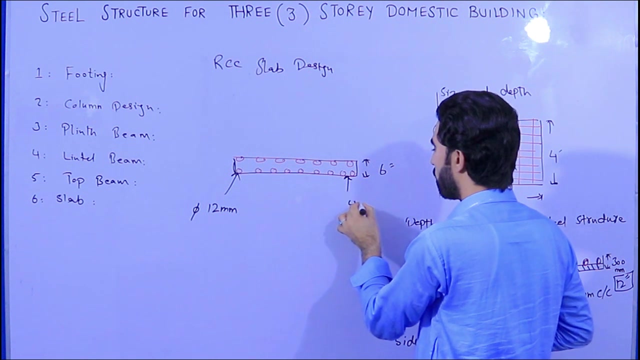 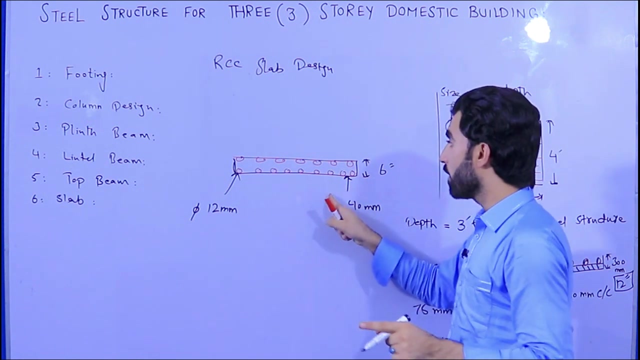 main bars and distribution bars. okay, and the dia of main bar and distribution bar: same main bar and distribution bar, dia was same, which was 12 millimeter, which was 12 millimeter. and concrete cover guys, it should be 40 mm. okay, but it should be 40 mm in the case of and the case of when the thickness of the slab is more than six inches. but 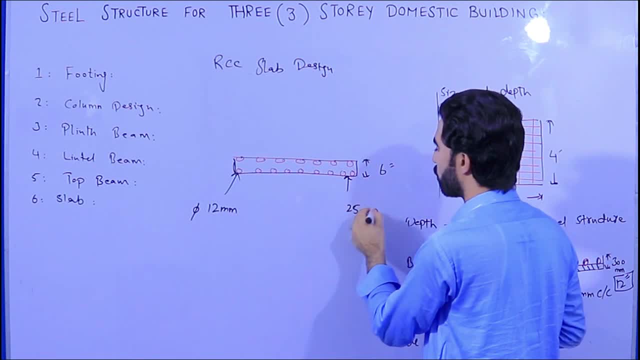 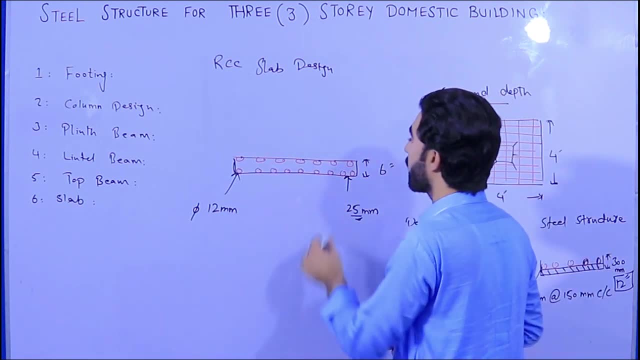 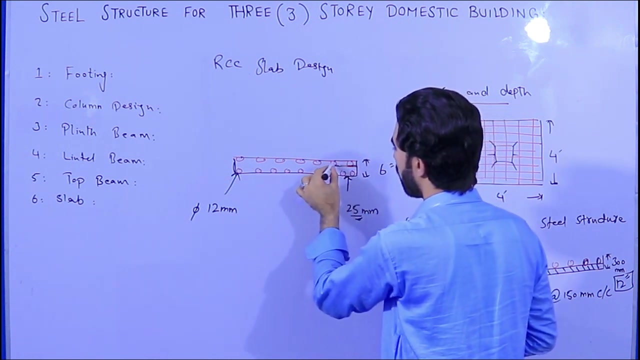 here I did with 25 mm, one inch top and bottom right concrete cover. and also, guys, we provide here crank bar. also here is crank bar. okay, that is this same like this crank bar, we also develop. and also here is crank bar. okay, that is this same like this crank bar, we also develop. 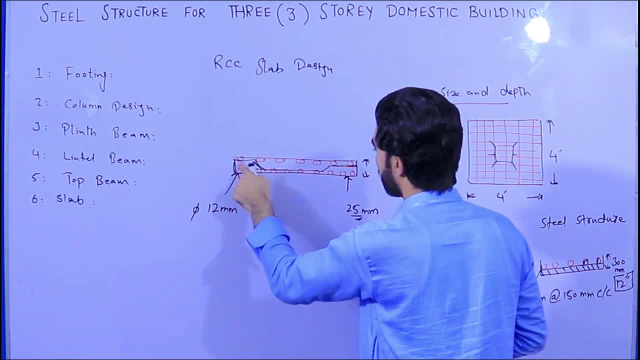 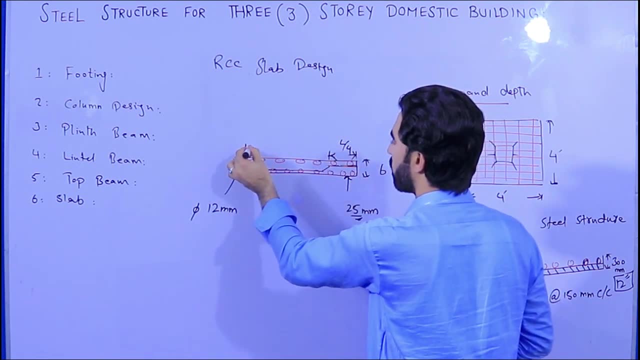 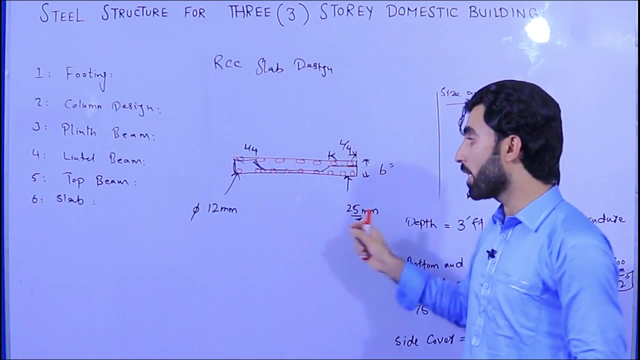 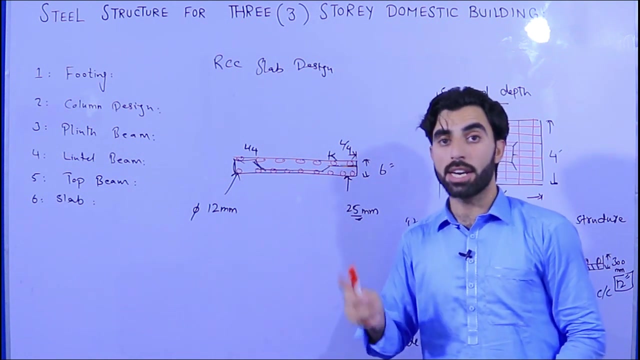 so ground in x. Мне sorry, okay. and the formula is L by 4, also L by 4. this is the steel structure design for RC C slave man bar distribution bar dia was 12 millimeter. and also we provide crank bar and the crank bar. 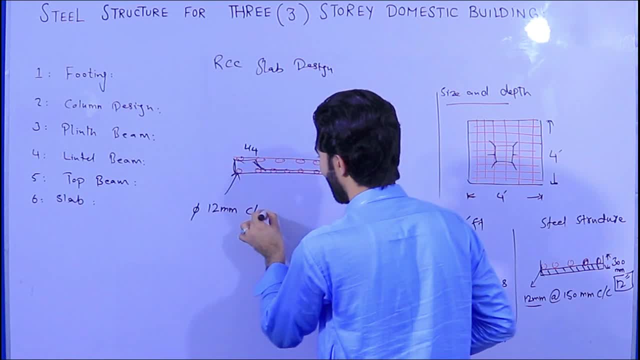 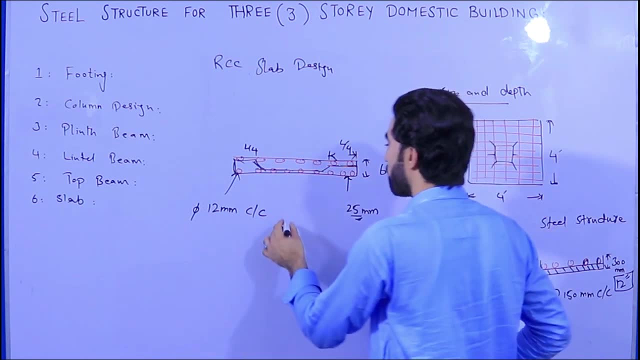 was the first steel bar main bars. then distribution bar was 12 mm range man bar. distribution bar was 12 distribution bar. sorry, with the spacing off. okay, so if I am NOT discussing these things so many students, they come in. sir, what is the spacing? the spacing was 150.